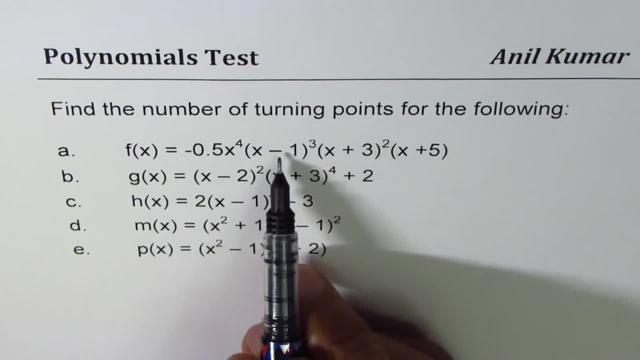 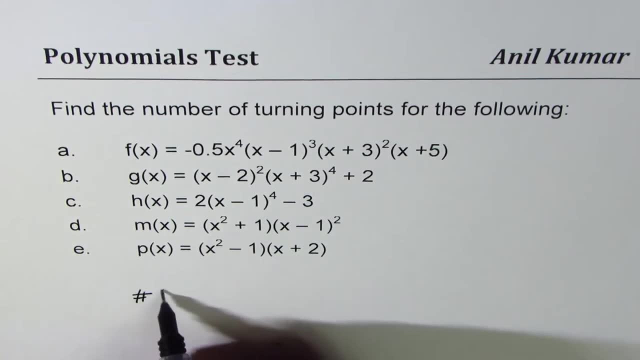 many. Number of turning points really depend on number of zeros and number of even zeros. Let me give you a formula here: Number of turning points is equal to number of zeros minus 1 plus number of even zeros. So we will use this formula to find number. 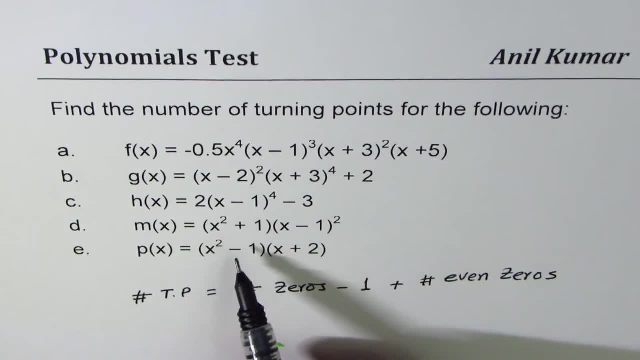 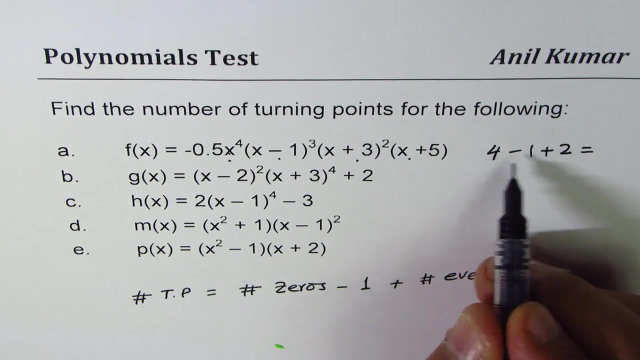 of turning points. You can always sketch these functions and figure out the answer. In the first one we have one, two, three, four zeros, So we get four zeros Minus one. and even zeros are one and one, two, So plus two, So that gives us four minus. 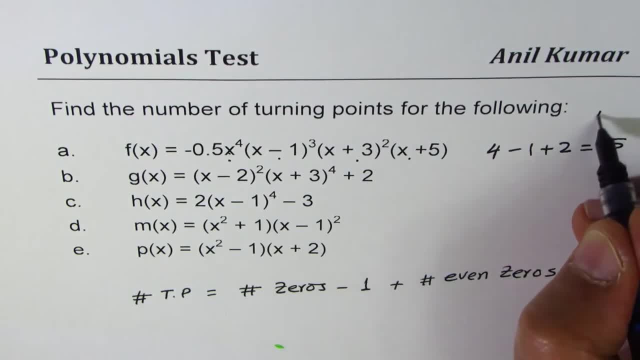 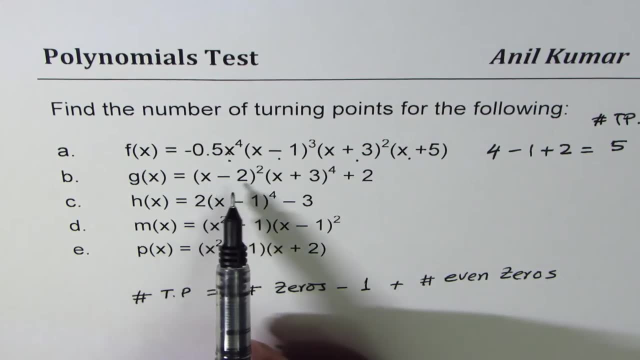 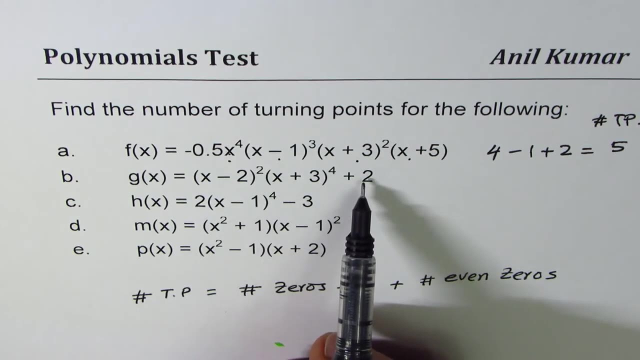 one is three, three plus two is five. So that is the number of turning points. The next one here is kind of tricky. What we have here is two zeros, but we are taking the function above. It doesn't really change the number of turning points, So we can still count them. 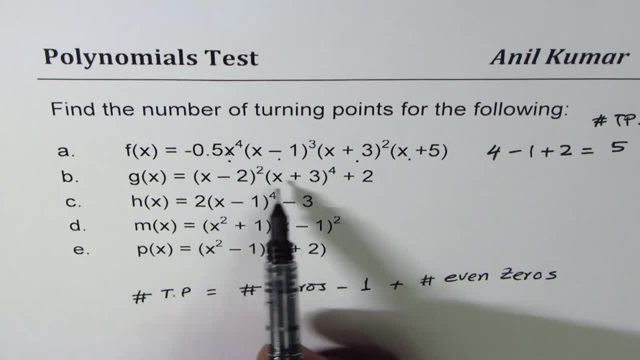 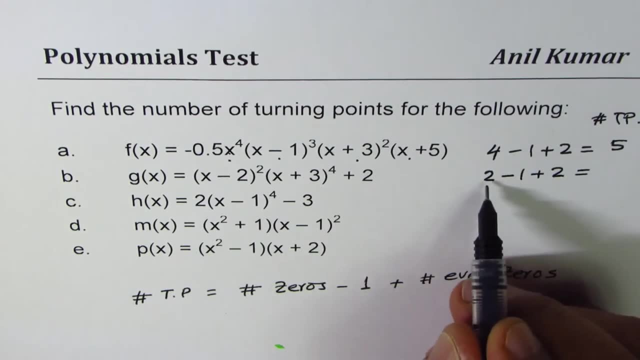 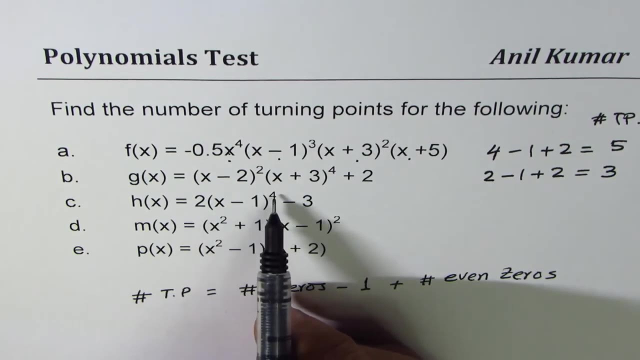 as zeros. right, So we have two zeros. Both of them are even, So the formula will be two minus one plus two, even zeros, And that gives us four minus one as three. Now in this case, we have x minus one to the power of four. The function is like a parabola which opens. 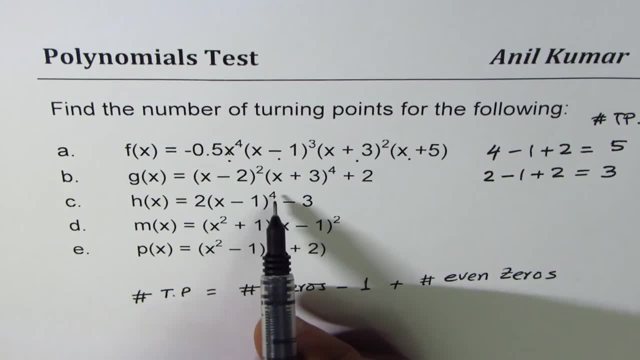 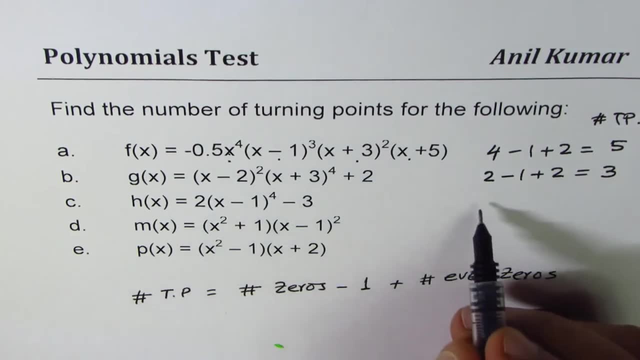 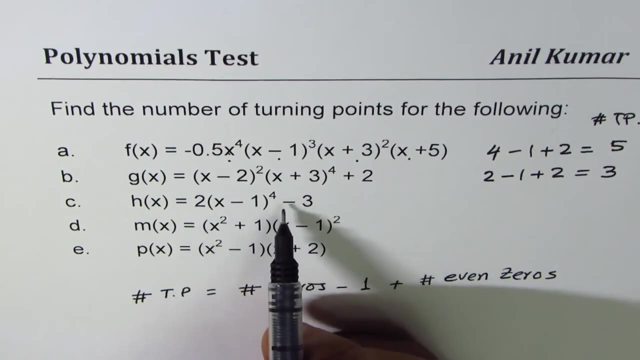 upwards with the equation, the form of a vertex form. So that gives you only one turning point, right? So this one is just one turning point. You could use a formula like this, Ignoring the term minus three, we have one zero minus one plus number of. 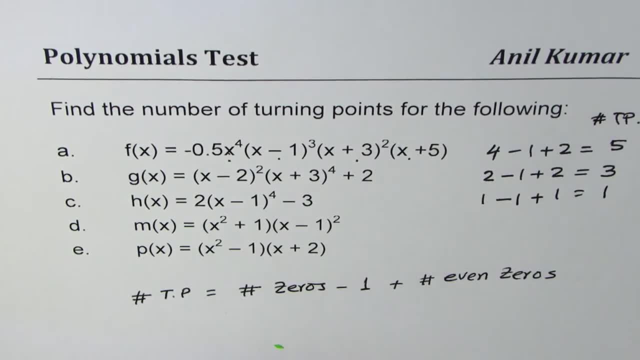 even zeros is one. So that gives us one turning point. Now here: x squared plus one is not a zero, not a real zero. X minus one is a zero. So we have one zero, Minus one for the minus one and plus one for a number of even zeros. So what we have